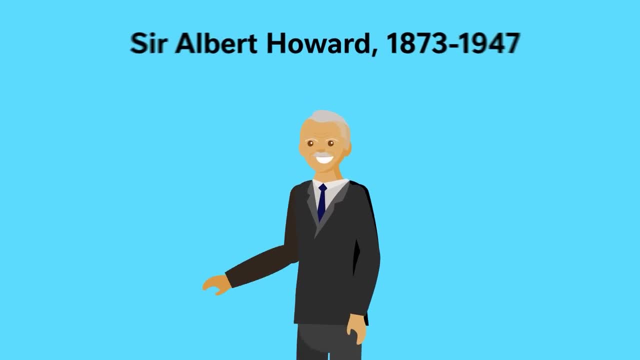 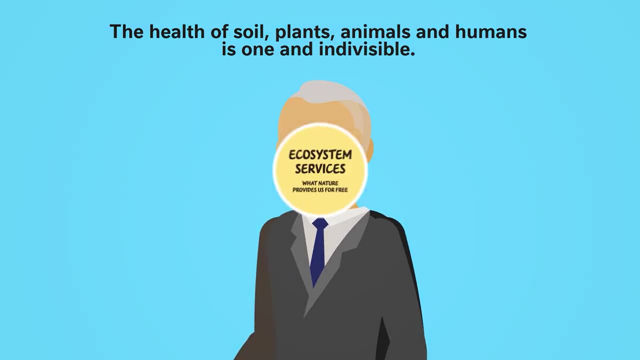 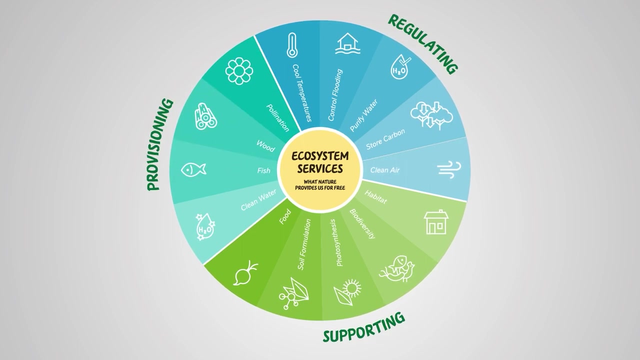 the UK, a founding father of organic agriculture. the health of soil plants, animals and humans is one and indivisible- были about 80% of the value of global ecosystem. services can be linked to soil functions Due to the diversity of soil processes. 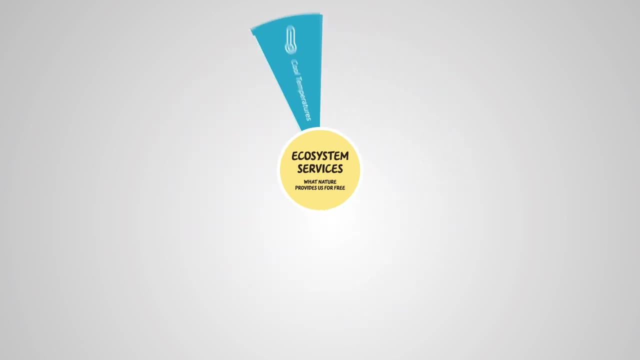 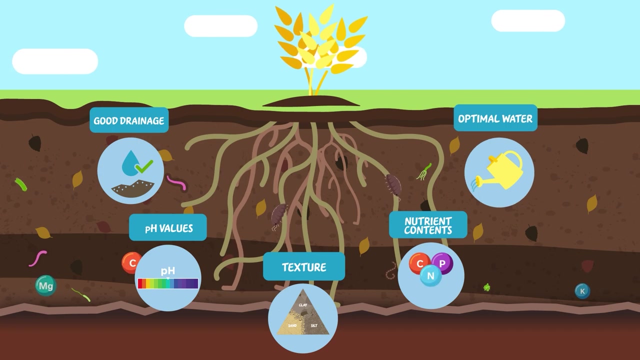 and of purposes soils are used for. soil health is not readily quantifiable, but there are common denominators. Most plants thrive best on soils with well-balanced properties. Soil should be stable, with no impenetrable layers in the root zone. 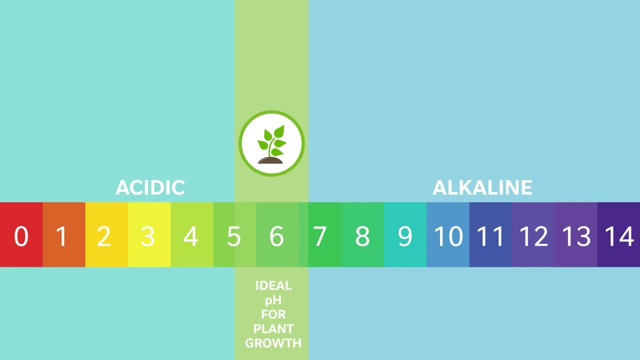 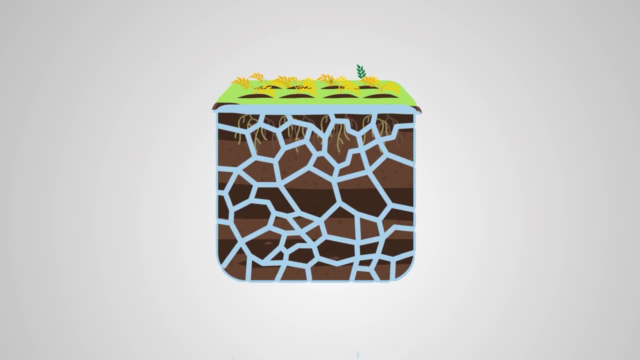 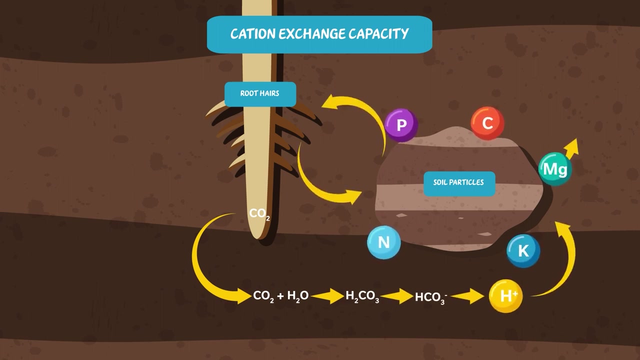 The pH should be slightly acidic to neutral, allowing for the uptake of metallic and alkaline nutrients. Moisture should be stored in sufficient quantities without water logging. The soil must be able to store nutrients, an ability measured via the cation exchange capacity. 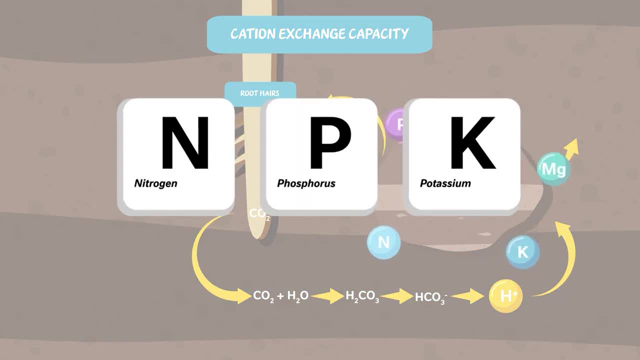 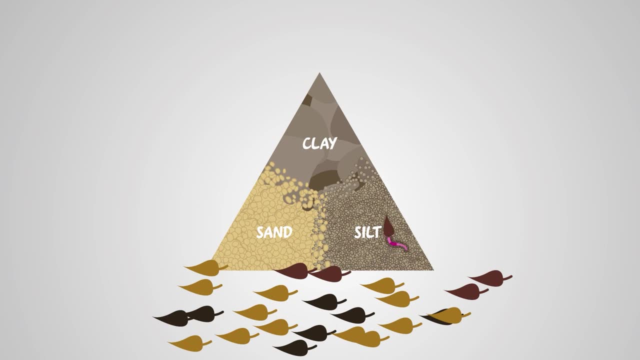 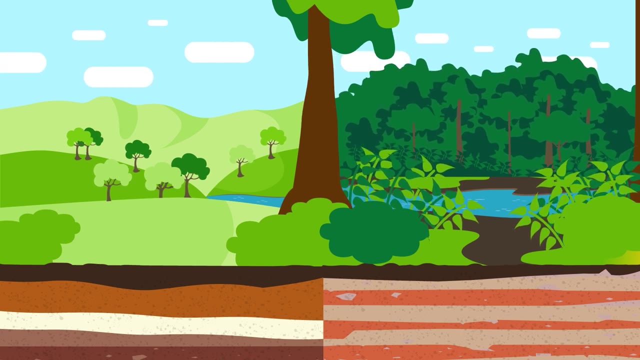 Essential nutrients like nitrogen, phosphorus and potassium must be sufficiently available to soil organisms and crops. Two keystones of soil health that mediate many of its aspects are soil texture and organic matter content. Some soil types have inherently favorable properties. Examples are the Black Earths and Temperate. 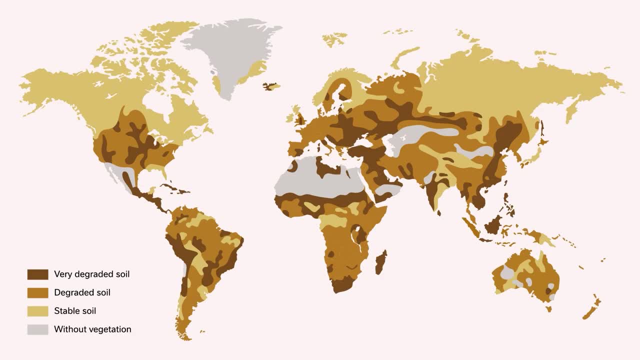 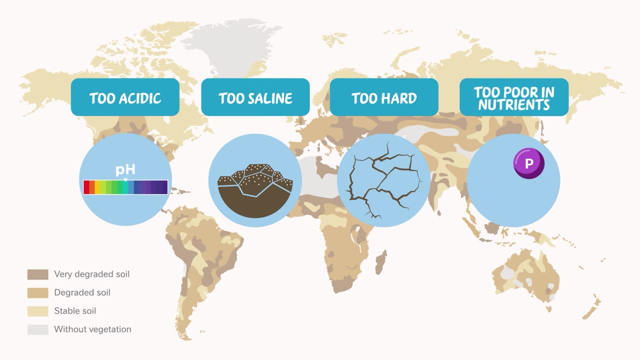 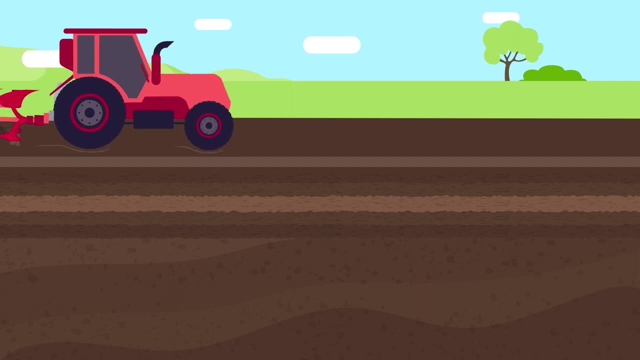 and Anisols in tropical ecozones. Much land is covered by problem soils: Too acidic or too saline, too unstable or too hard, too poor in nutrients or organic matter for optimal plant growth. On top of that, we continue to lose some of our best agricultural lands. 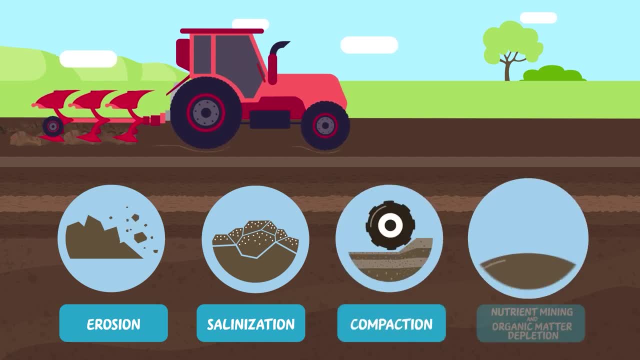 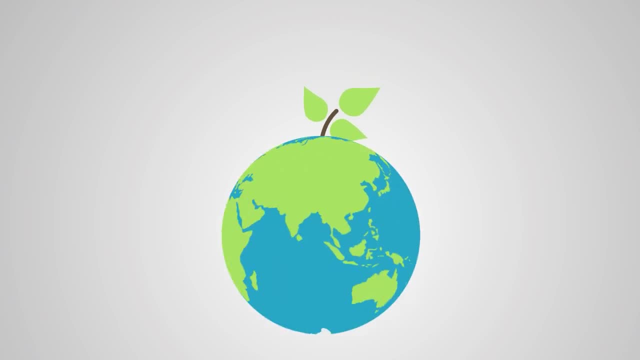 due to erosion, salinization, compaction, nutrient mining and expansion and other processes of land degradation. By keeping soils healthy, farmers fulfill an essential task and act as trustees of humankind. 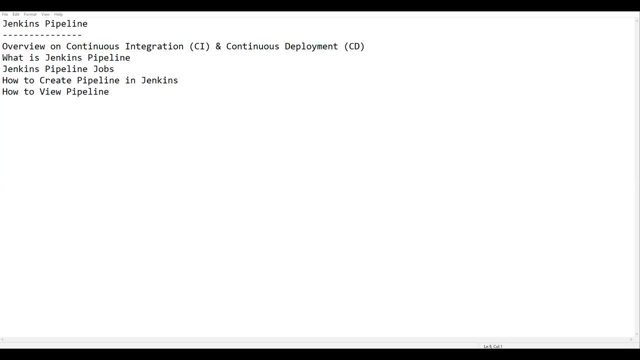 hi everyone, welcome you all. in this video, I'm going to talk about a topic called Jenkins pipeline. so this topic is very important for especially as dead engineers as well as DevOps engineers. so let's see what it is. so, Jenkins pipeline. so, before understanding what is exactly Jenkins pipeline, we need to know. 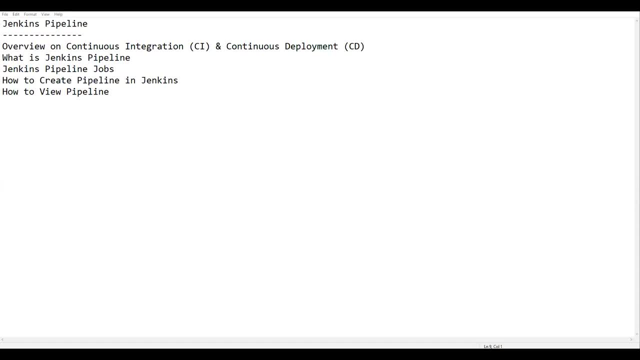 very basic concept of continuous integration, continuous deployment. so first let us start with the continuous integration, continuous deployment and then we'll come back and discuss about the Jenkins pipeline, all right, so first of all let me just talk about CI and CD processes, continuous integration, continuous development. so normally when you're working on any projects or it can,